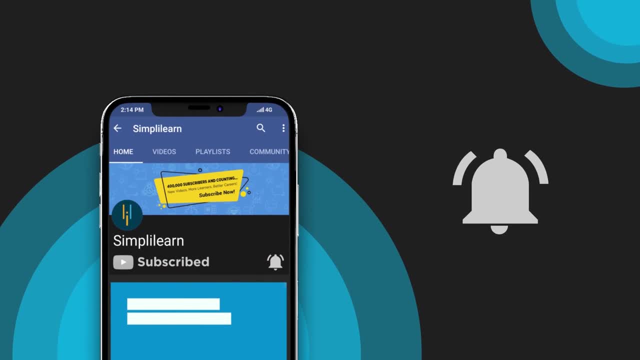 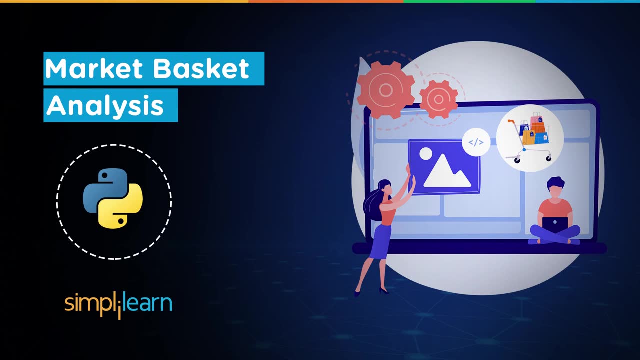 Hello everyone, I am Mayank and welcome to Simply Learn. Today we will take you through the hands-off lab demo of how you can do a market basket analysis using Python. Before we start, I hope the screen is clearly visible and the audio is fine. If yes, please type. 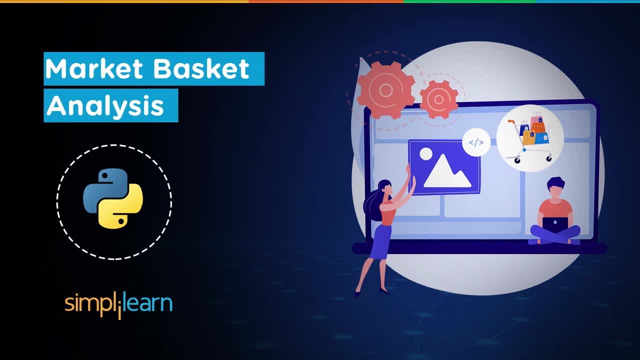 in yes. If there are any issues, do let us know in the chat section so that we can resolve them. I am repeating again before we start. I hope the screen is clearly visible and the audio is fine. If yes, please type in yes. If there are any issues, do let us know in. 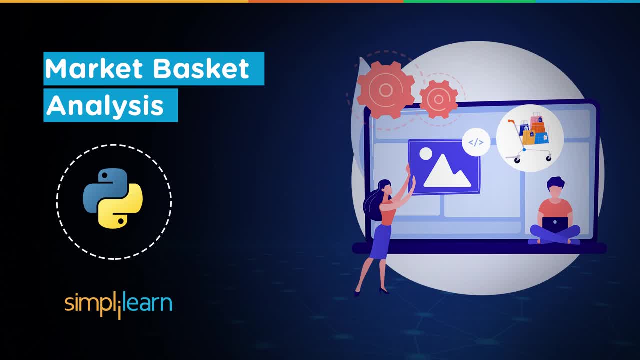 the chat section so that we can resolve them. Let's wait for some more minutes to let other people join. Until then, let me tell you guys that we have regular updates on multiple technologies. If you are a tech geek on a continuous hunt for the latest technological trends, then 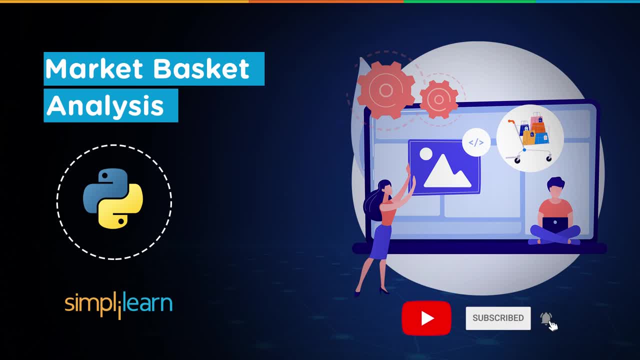 consider getting subscribed to our YouTube channel and press that bell icon. I'm repeating again before we start. I hope the screen is clearly visible and the audio is fine. After that you can test this demo. Let's wait for some more minutes to let other 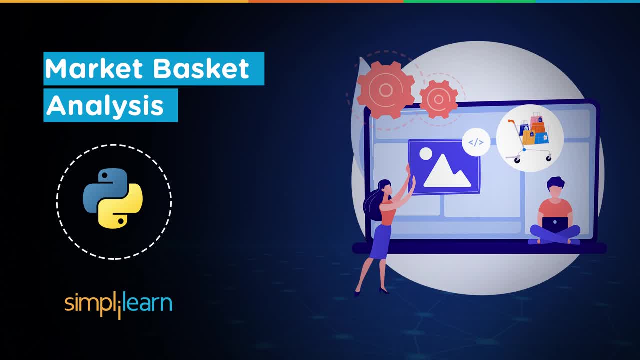 people join. Until then, let's wait for some more minutes to let other people join. I am repeating again before we start. I hope the screen is clearly visible and the audio is fine If you are a tech geek on a continuous hunt for the latest technological trends. 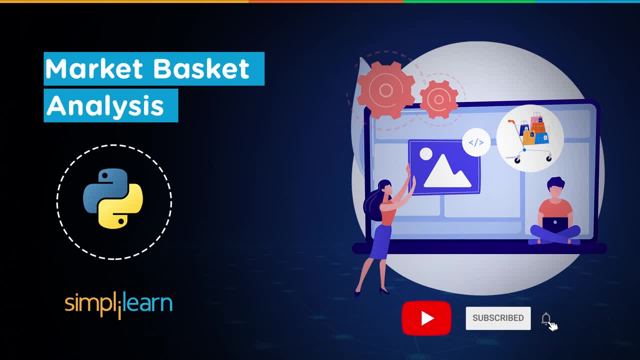 then consider getting subscribed to our YouTube channel and press that bell icon你就 nie macam Sentinel kamu Hokut panels Presen yang dapat dikat, And I hope the screen is clear. After that you can test this demo and also during our conversation we can. 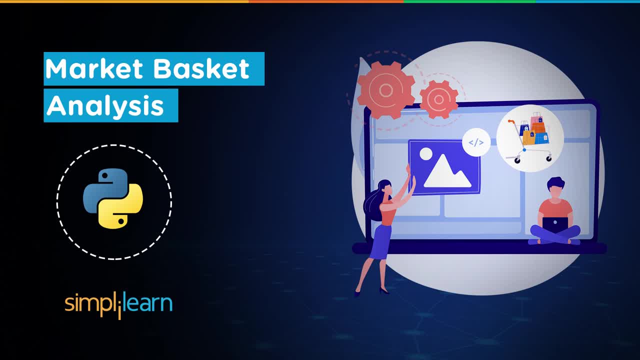 demonstrate the strens. In today's session we will go through market basket analysis. after that, a hands off lab demo of market basket analysis will be done using Python. Market basket analysis will be done using Python and machine learning. We will perform different functions and different Python libraries. 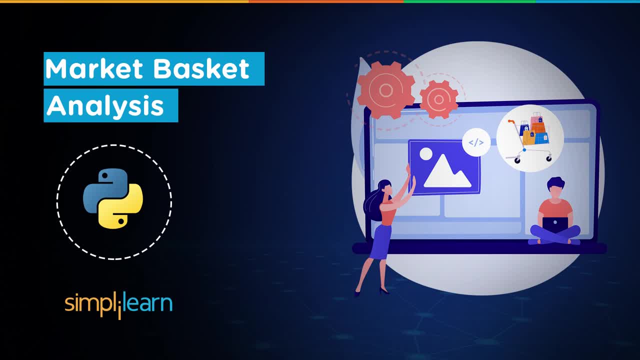 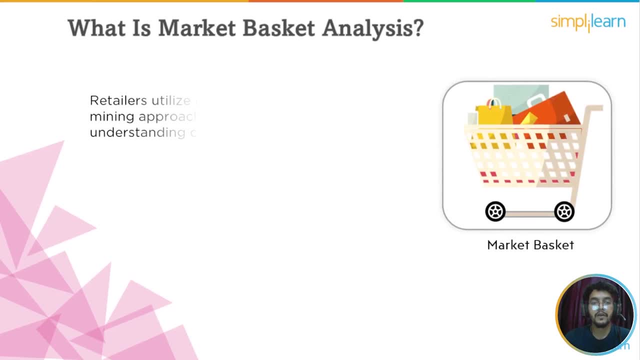 Before we move on to the programming part, let's discuss what market basket analysis first and proceed further for the same. What is market basket analysis? Retailers utilize market basket analysis, a data mining approach, to boost sales by better understanding client-bind patterns. 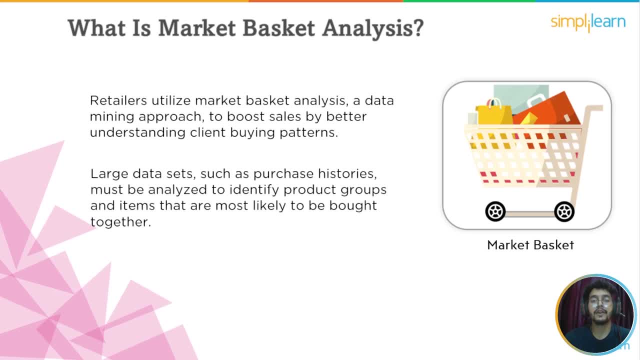 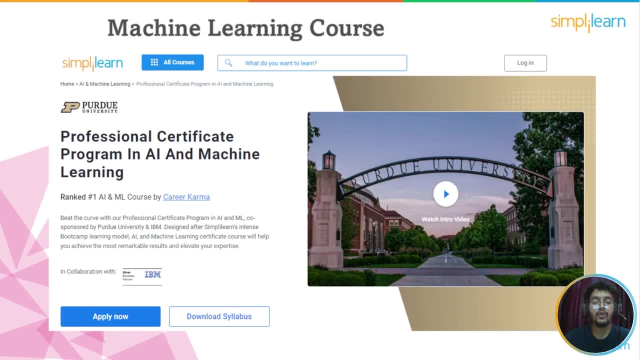 Part. data sets, such as purchase histories, must be analyzed to identify products, groups and items that are most likely to be bought together. So, dear learners, if you want to upskill your AI and machine learning skills, so give yourself a chance to simply learn profession certificate program in AI and machine learning, which 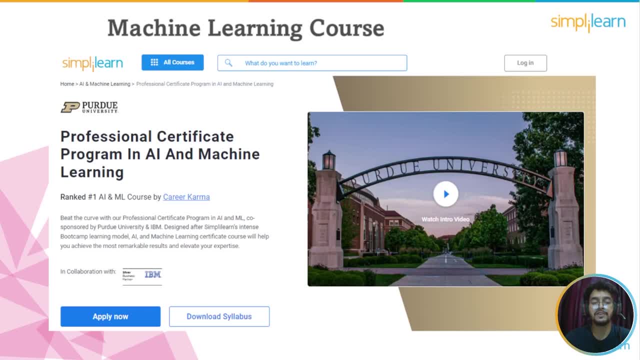 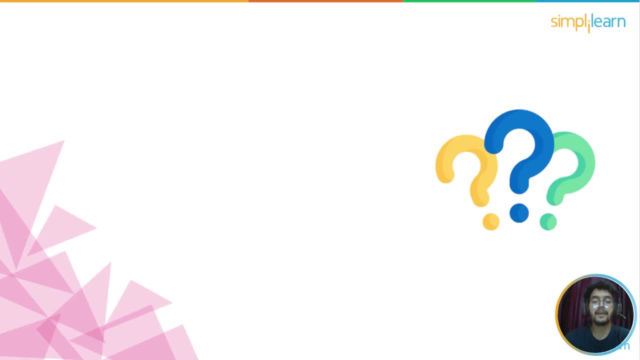 comes with completion certificate and in-depth knowledge of AI and machine learning. check this course details from the description box below. So here is one question for you guys. I will give you exactly one minute for this. You can comment or you can give your answer in the chat section so I can see if the answer. 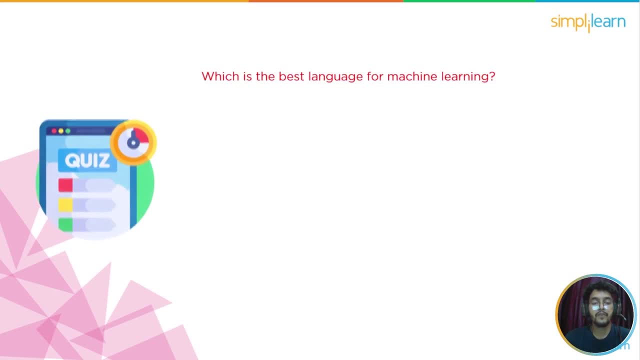 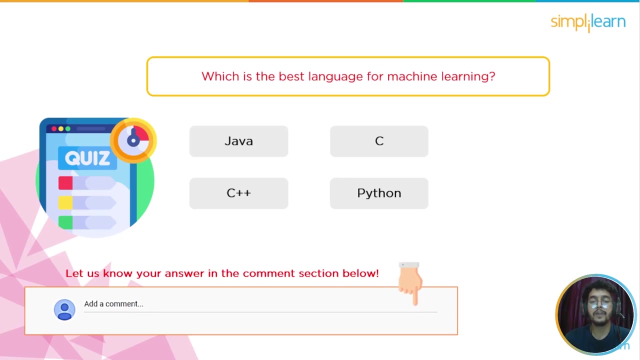 is given by you are right or wrong. So the question is: which is the best language for machine learning- Java, C, C++, Python. Let us know your answer in the comment section or in the chat section? Do let me know your answer, please. 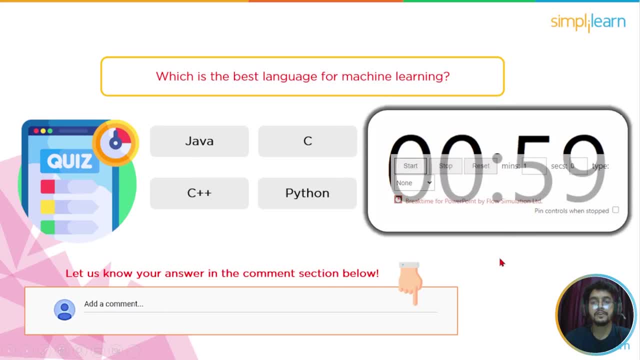 So I am starting timer of one minute, So your time starts now. Which is the best language for machine learning? Java, C, C++ or Python? You can type your answer in the comment section or in the chat section. Do let me know your answer, please. 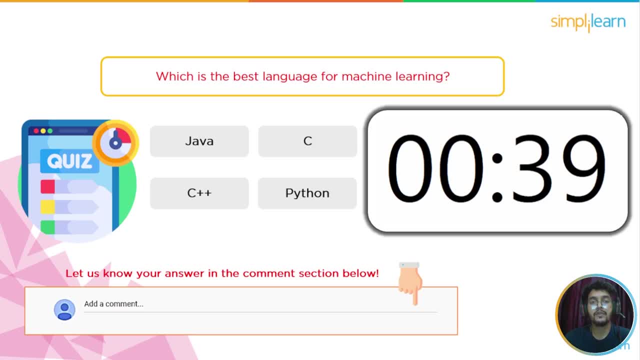 I kindly ask that everyone should take part in this. Which is the best language for machine learning? Java, C, C++ or Python? Thirty seconds more. Let us know your answer in the comment section. Which is the best language for machine learning? Java, C, C++ or Python? 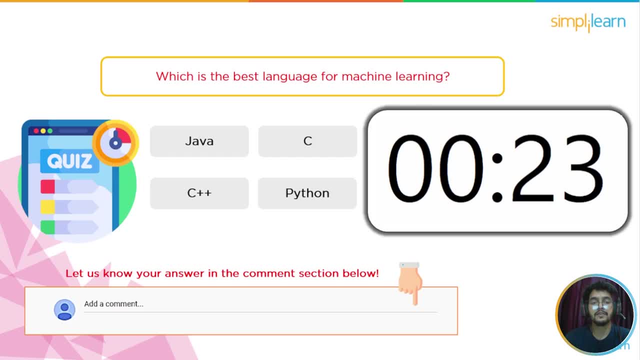 Fifteen seconds more. Which is the best language for machine learning? Java, C, C++ or Python? I kindly ask that everyone should take part in this. Fifteen seconds more. Which is the best language for machine learning? Java, C, C++ or Python? 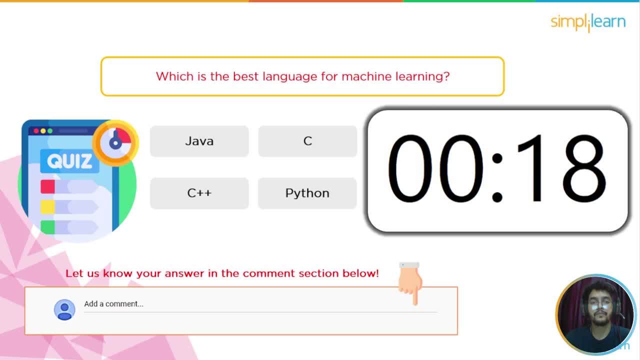 Fifteen seconds more. Which is the best language for machine learning? Java, C, C++ or Python? I kindly ask that everyone should take part in this. Fifteen seconds more. Which is the best language for machine learning? Java, C, C++ or Python? 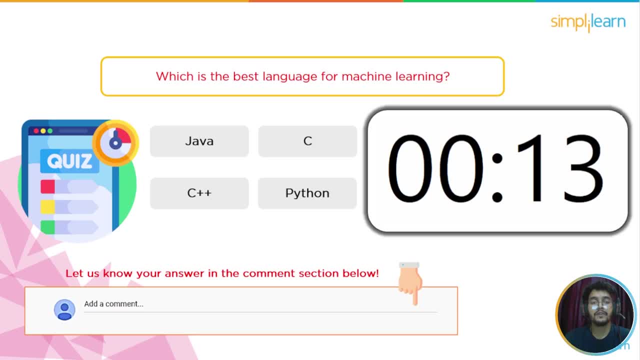 Fifteen seconds more. Which is the best language for machine learning? Java, C, C++ or Python? I kindly ask that everyone should take part in this. Fifteen seconds more. Which is the best language for machine learning? Java, C, C++ or Python? 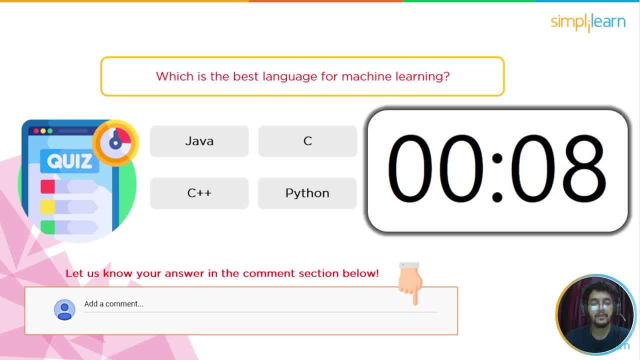 I kindly ask that everyone should take part in this Fifteen seconds more. Which is the best language for machine learning? Java, C, C++ or Python? I kindly ask that everyone should take part in this Fifteen seconds more. Which is the best language for machine learning? Java, C, C++ or Python? 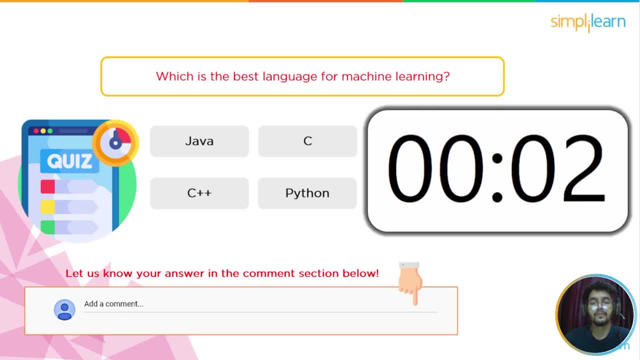 I kindly ask that everyone should take part in this. Fifteen seconds more. Which is the best language for machine learning? Java, C, C++ or Python? Fifteen seconds more. Which is the best language for machine learning? Java, C, C++ or Python? 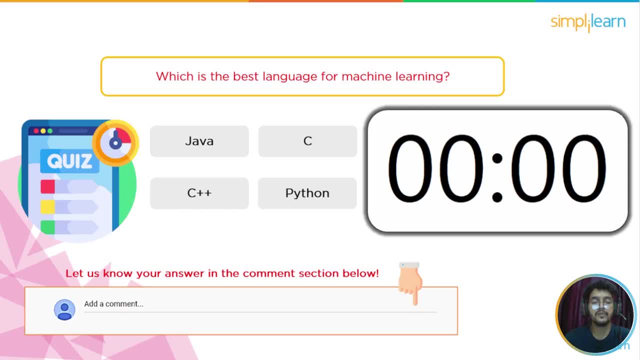 I kindly ask that everyone should take part in this Fifteen seconds more. Which is the best language for machine learning? Java, C, C++ or Python? I kindly ask that everyone should take part in this Fifteen seconds more. Which is the best language for machine learning? Java, C, C++ or Python? 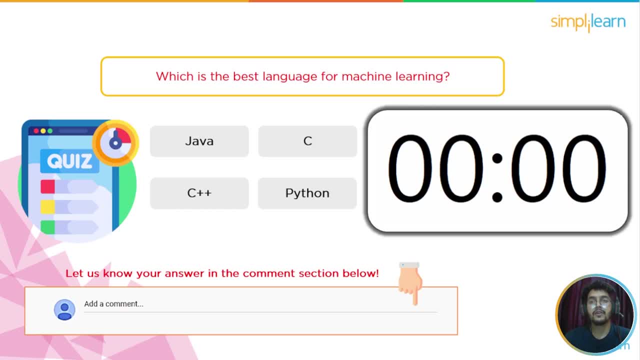 I kindly ask that everyone should take part in this Fifteen seconds more. Which is the best language for machine learning? Java, C, C++ or Python? I kindly ask that everyone should take part in this Fifteen seconds more. Which is the best language for machine learning? Java, C, C++ or Python? 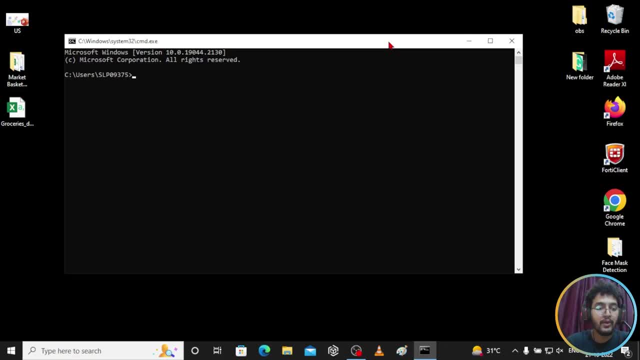 I kindly ask that everyone should take part in this Fifteen seconds more. Which is the best language for machine learning? Java, C, C++ or Python? I kindly ask that everyone should take part in this Fifteen seconds more. Which is the best language for machine learning? Java, C, C++ or Python? 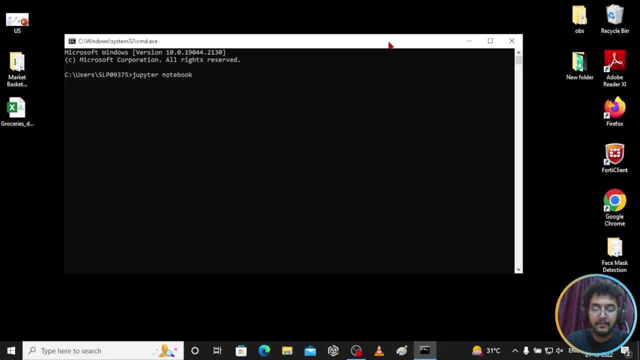 I kindly ask that everyone should take part in this Fifteen seconds more. Which is the best language for machine learning? Java, C, C++ or Python? I kindly ask that everyone should take part in this Fifteen seconds more. Which is the best language for machine learning? Java, C, C++ or Python? 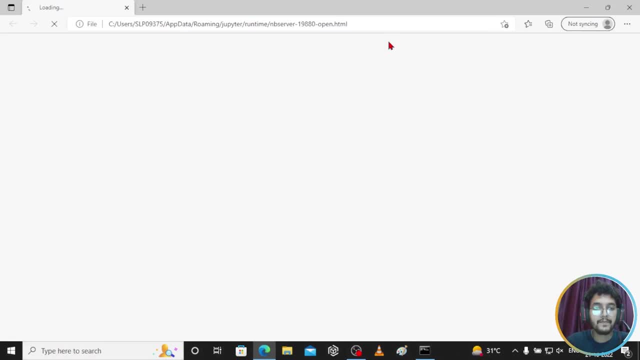 I kindly ask that everyone should take part in this Fifteen seconds more. Which is the best language for machine learning? Java, C, C++ or Python? I kindly ask that everyone should take part in this Fifteen seconds more. Which is the best language for machine learning? Java, C, C++ or Python? 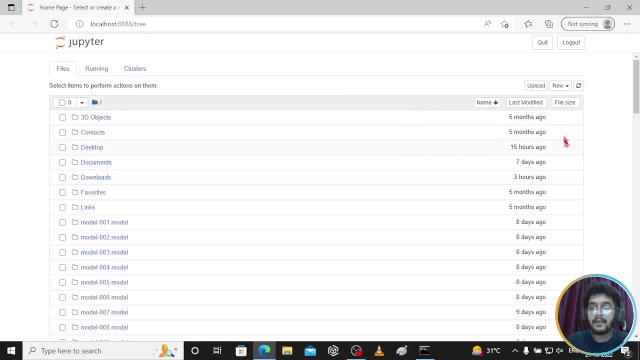 I kindly ask that everyone should take part in this Fifteen seconds more. Which is the best language for machine learning? Java, C, C++ or Python? I kindly ask that everyone should take part in this Fifteen seconds more. Which is the best language for machine learning? Java, C, C++ or Python? 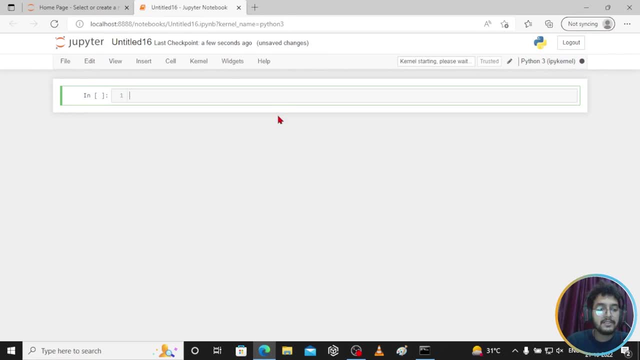 I kindly ask that everyone should take part in this Fifteen seconds more. Which is the best language for machine learning? Java, C, C++ or Python? I kindly ask that everyone should take part in this Fifteen seconds more. Which is the best language for machine learning? Java, C, C++ or Python? 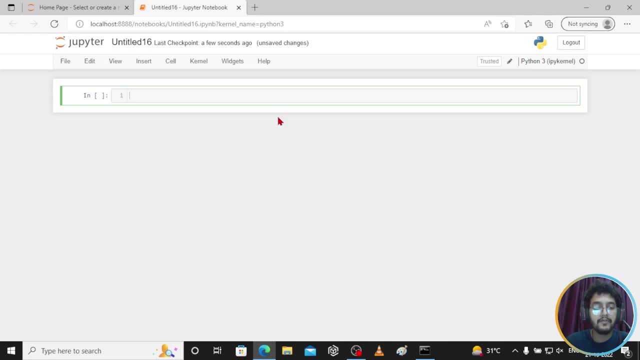 I kindly ask that everyone should take part in this Fifteen seconds more. Which is the best language for machine learning? Java, C, C++ or Python? I kindly ask that everyone should take part in this Fifteen seconds more. Which is the best language for machine learning? Java, C, C++ or Python? 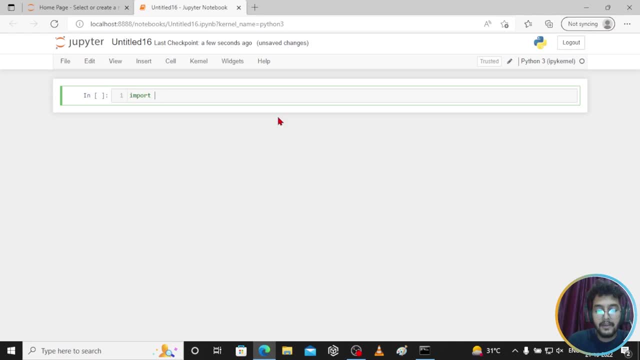 I kindly ask that everyone should take part in this Fifteen seconds more. Which is the best language for machine learning? Java, C, C++ or Python? I kindly ask that everyone should take part in this Fifteen seconds more. Which is the best language for machine learning? Java, C, C++ or Python? 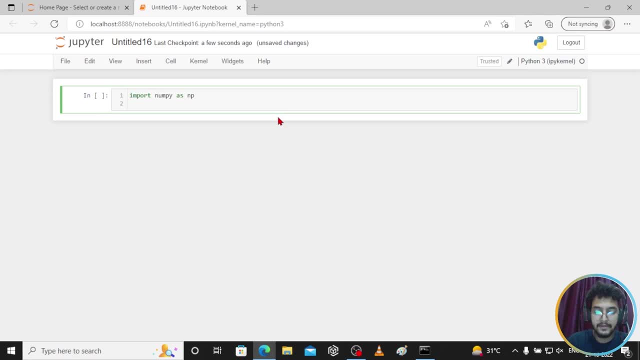 I kindly ask that everyone should take part in this Fifteen seconds more. Which is the best language for machine learning? Java, C, C++ or Python? I kindly ask that everyone should take part in this Fifteen seconds more. Which is the best language for machine learning? Java, C, C++ or Python? 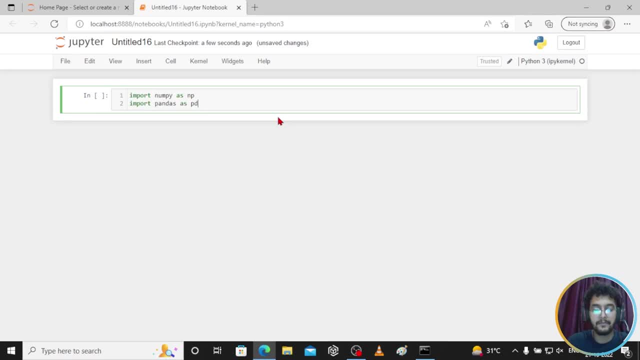 I kindly ask that everyone should take part in this Fifteen seconds more. Which is the best language for machine learning? Java, C, C++ or Python? I kindly ask that everyone should take part in this Fifteen seconds more. Which is the best language for machine learning? Java, C, C++ or Python? 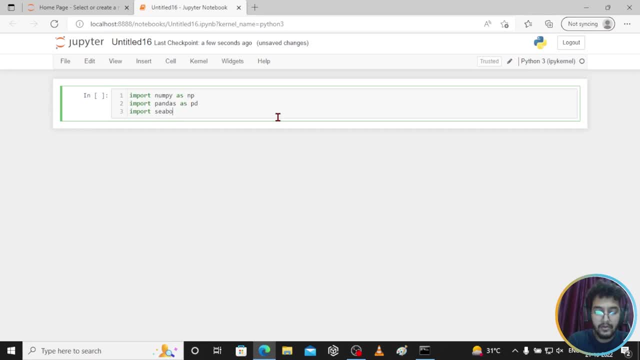 I kindly ask that everyone should take part in this Fifteen seconds more. Which is the best language for machine learning? Java, C, C++ or Python? I kindly ask that everyone should take part in this Fifteen seconds more. Which is the best language for machine learning? Java, C, C++ or Python? 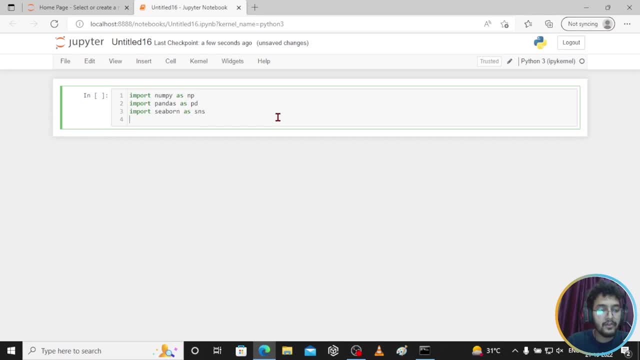 I kindly ask that everyone should take part in this Fifteen seconds more. Which is the best language for machine learning? Java, C, C++ or Python? I kindly ask that everyone should take part in this Fifteen seconds more. Which is the best language for machine learning? Java, C, C++ or Python? 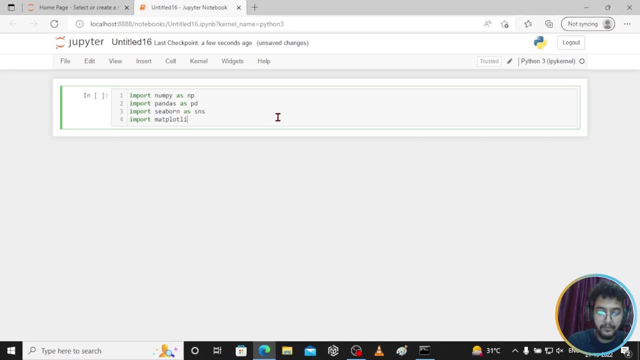 I kindly ask that everyone should take part in this Fifteen seconds more. Which is the best language for machine learning? Java, C, C++ or Python? I kindly ask that everyone should take part in this Fifteen seconds more. Which is the best language for machine learning? Java, C, C++ or Python? 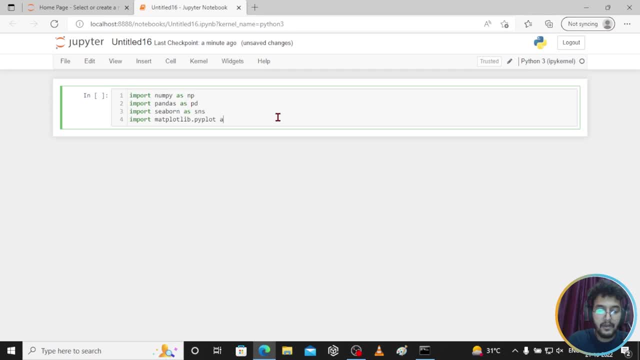 I kindly ask that everyone should take part in this Fifteen seconds more. Which is the best language for machine learning? Java, C, C++ or Python? I kindly ask that everyone should take part in this Fifteen seconds more. Which is the best language for machine learning? Java, C, C++ or Python? 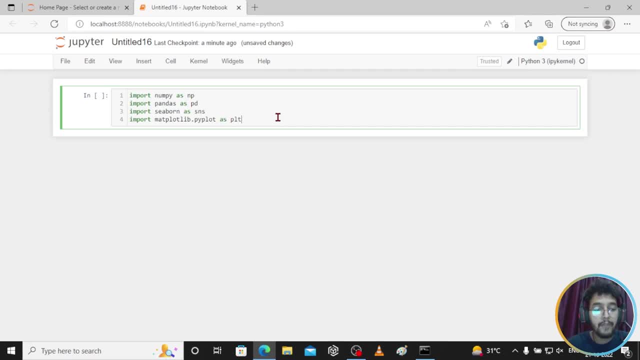 I kindly ask that everyone should take part in this Fifteen seconds more. Which is the best language for machine learning? Java, C, C++ or Python? I kindly ask that everyone should take part in this Fifteen seconds more. Which is the best language for machine learning? Java, C, C++ or Python? 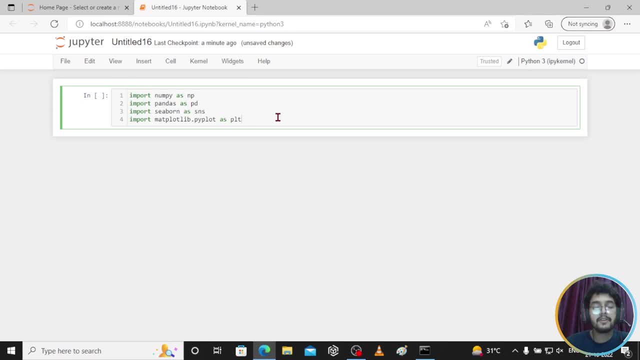 I kindly ask that everyone should take part in this Fifteen seconds more. Which is the best language for machine learning? Java, C, C++ or Python? I kindly ask that everyone should take part in this Fifteen seconds more. Which is the best language for machine learning? Java, C, C++ or Python? 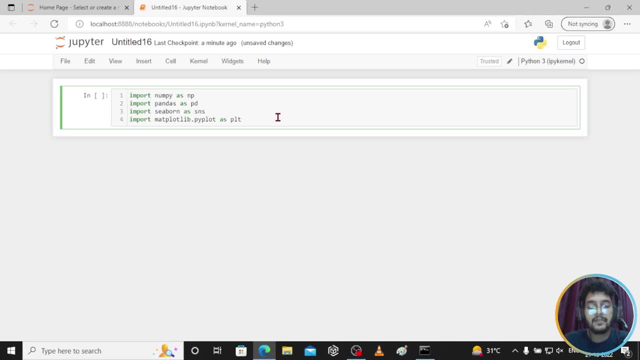 I kindly ask that everyone should take part in this Fifteen seconds more. Which is the best language for machine learning? Java, C, C++ or Python? I kindly ask that everyone should take part in this Fifteen seconds more. Which is the best language for machine learning? Java, C, C++ or Python? 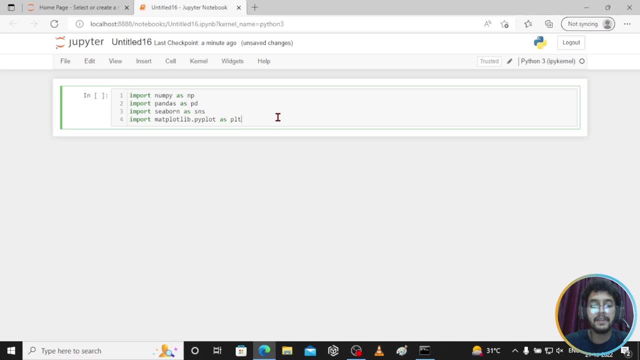 I kindly ask that everyone should take part in this. Fifteen seconds more. Which is the best language for machine learning? Java, C++ or Python? I kindly ask that everyone should take part in this. Which is the best language for machine learning? Java, C, C++ or Python? 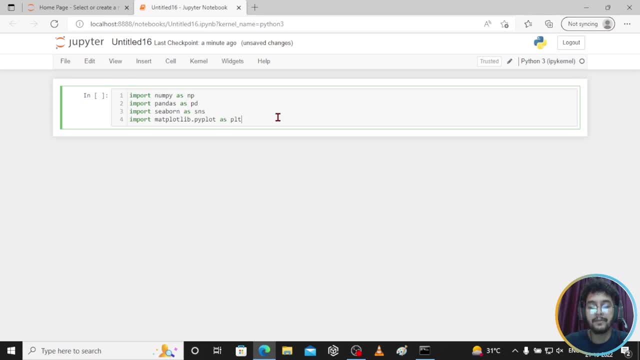 I kindly ask that everyone should take part in this, Either in simple сист dyed language or simple, or just if required. Do you want to know what called C, based on Matplotlib, is called Seaborn. It is utilized for data exploration and data. 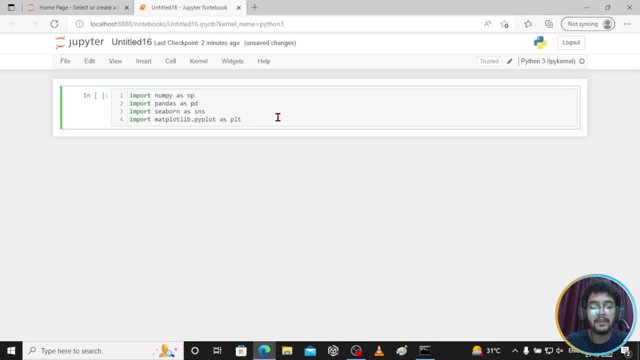 visualization With DataFrames and the Pandas library. Seaborn functions with ease For Python and its numerical extension, NumPy. Matplotlib is a cross-platform for data visualization and GUI. As a result, it represents a strong open source suitable for MATLAB. The API for 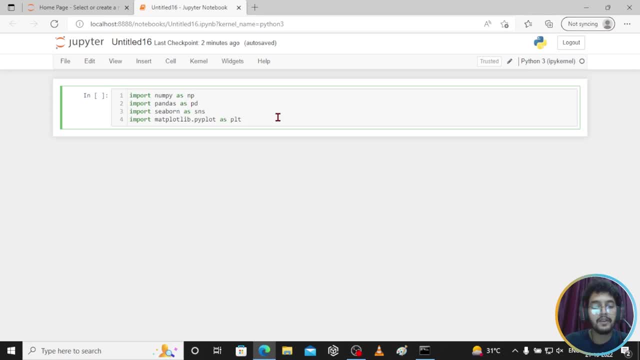 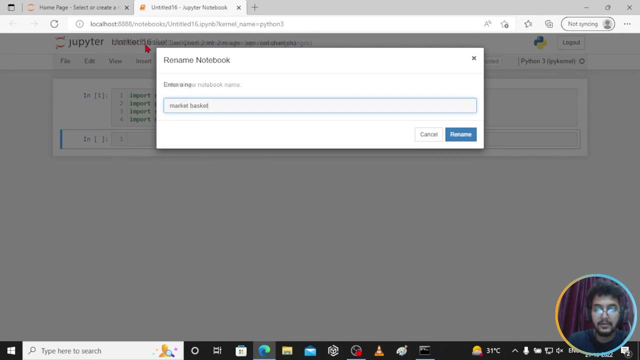 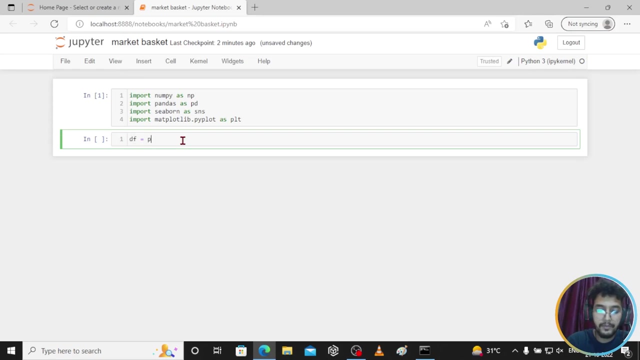 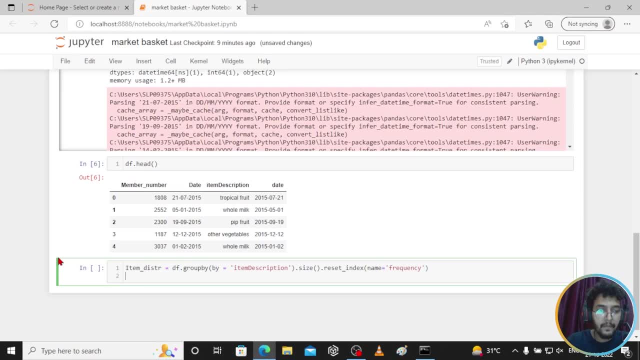 Okay, so here I will rename this market basket. Okay, so here I will rename this market basket. okay, i will write here dot. sort underscore values by frequency. frequency: okay, here f is also capital. then in ascending order, ascending equals to false. and here i will write dot head. 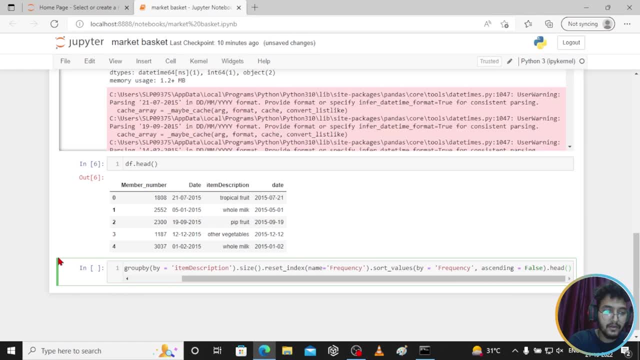 then here i will give 10, okay, then enter. so now i will declare some variables. so here i will write: bars equals to item underscore distribution. okay, then item description. okay, then height. equals to item underscore distribution. okay, then here. frequency, then item x underscore for position equals to np dot margin. 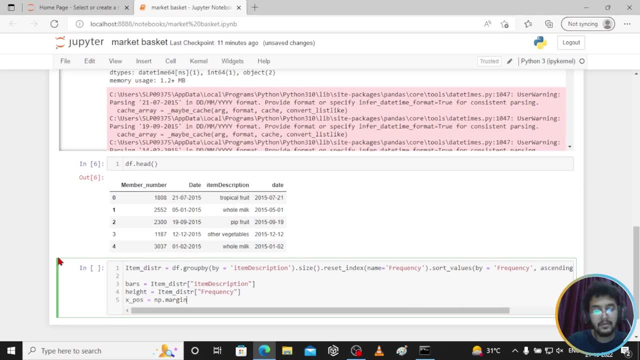 x underscore for position equals to np dot margin. uh, okay, not margin, i will write here. uh okay, not margin, i will write here. uh, okay, not margin, i will write here, arrange, arrange, arrange then. length of bars. length of then. length of bars. length of then. length of bars. length of bars. 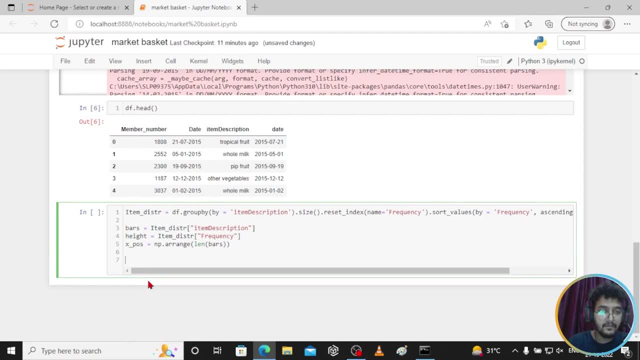 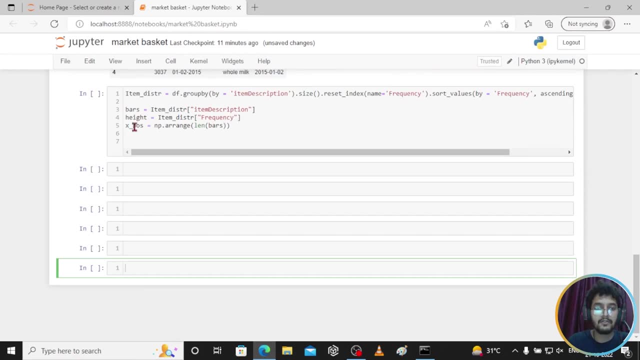 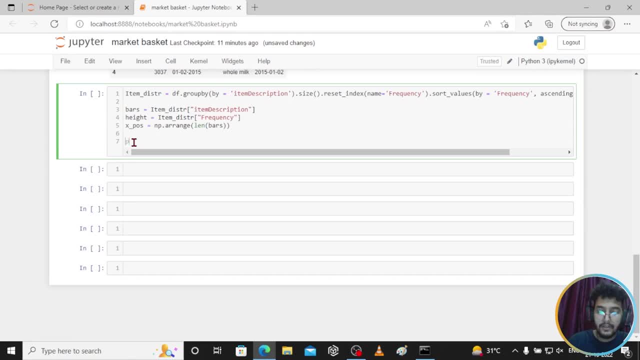 yeah, that's good. yeah, that's good. okay, so we will define here figure size. okay, so we will define here figure size. okay, so we will define here figure size. so for that i will write plt dot figure. so for that i will write plt dot figure. so for that i will write plt dot figure, then figure size. 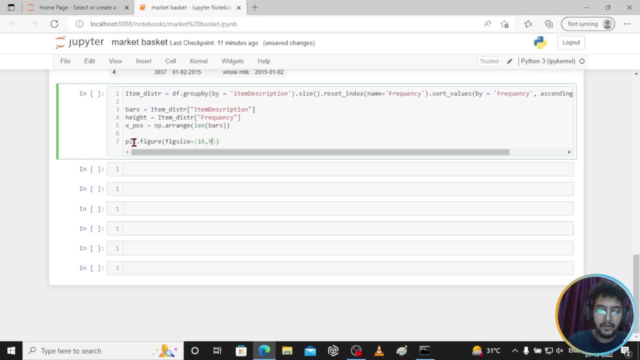 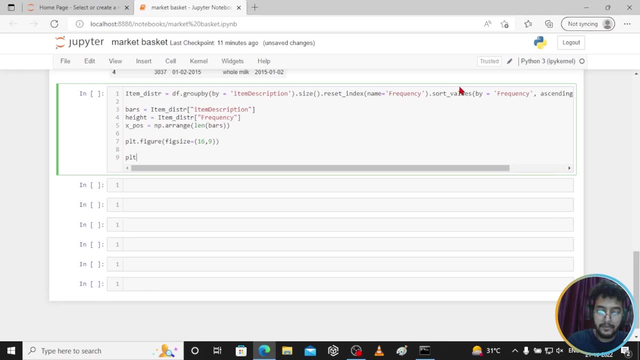 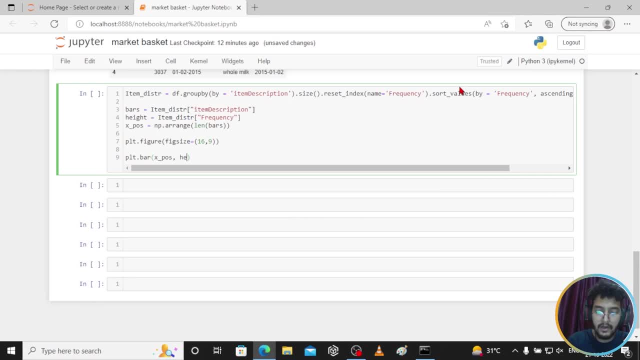 bar bar x. position x position x position: comma height: comma height. comma height: comma color: collect was to collect, was to collect was to. here i will do 0.2, here i will do 0.2, here i will do 0.2 comma 0.3. 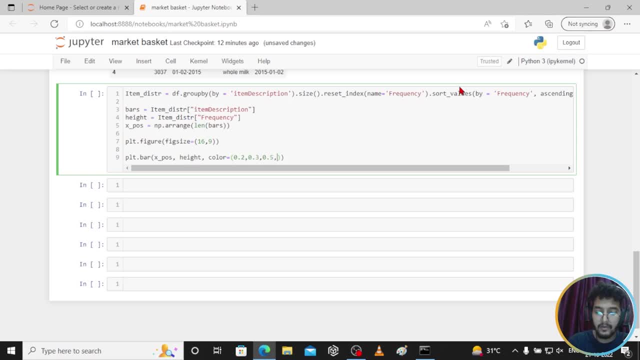 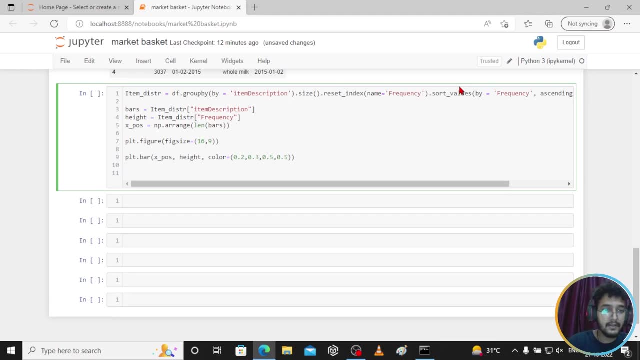 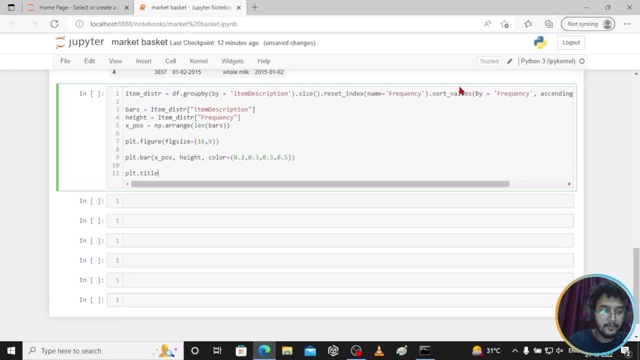 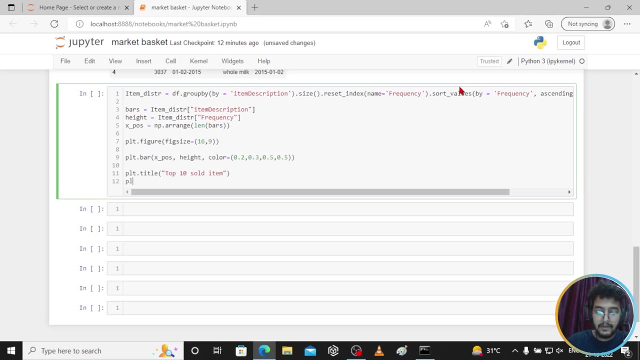 everything is done. let me set the title. so everything is done. let me set the title: plt dot, plt dot, plt dot title title title: like, like like top top, top then sold, then sold, then sold item item item then x label plt dot then x label plt dot. 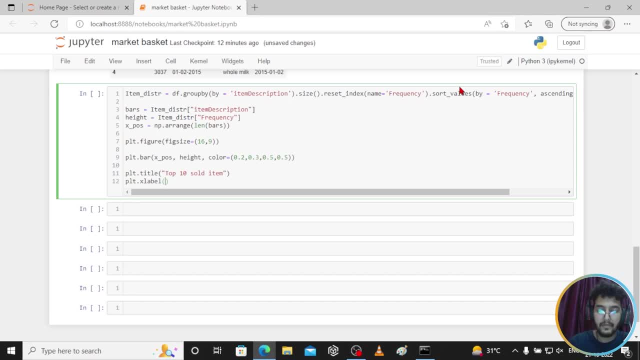 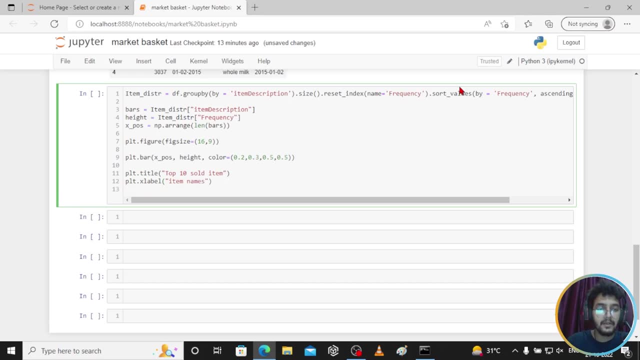 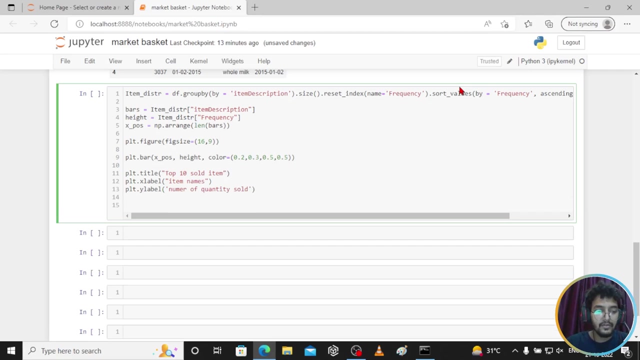 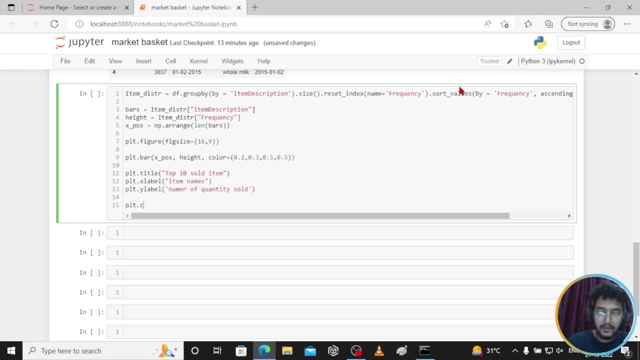 okay, so let me do plt dot. okay, so let me do plt dot. okay, so let me do the first step. okay, so let me do the first step. okay, so let me do the first step. okay, so like, create names on the like x-axis: okay, x sticks. 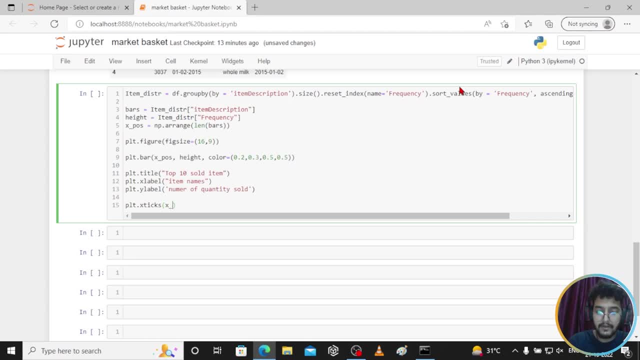 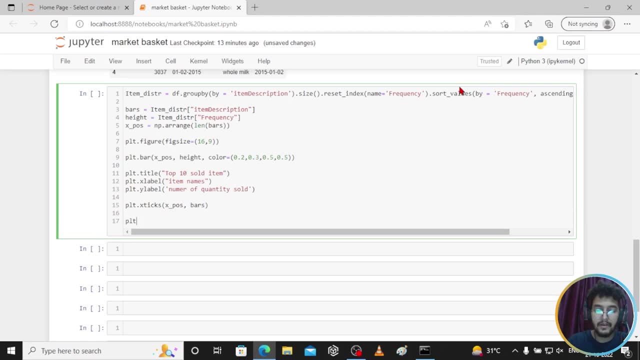 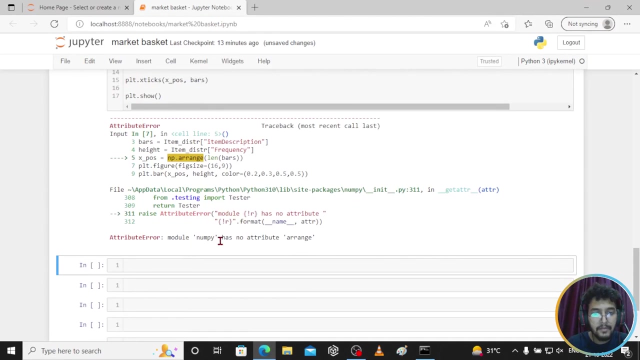 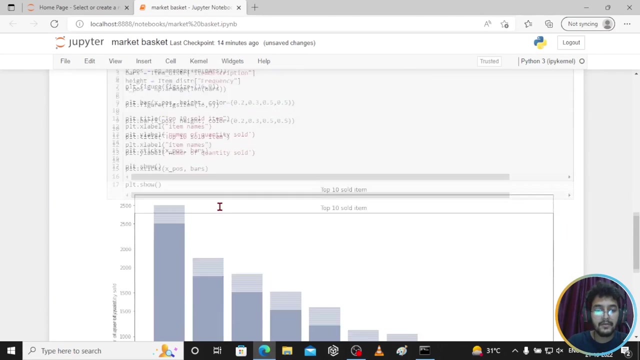 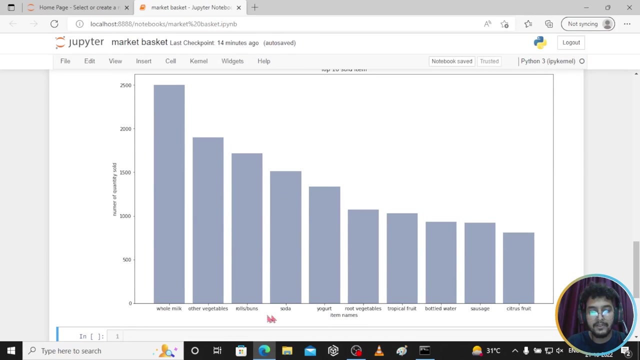 then x underscore position, comma bars. okay, then plt dot show. so then press enter. okay, np. arrange numpy has no attribute as arrange. okay, here is spelling mistake, so sorry. yeah, so here you can see the top 10 sold item. first the whole: make other vegetable rolls and burn soda. 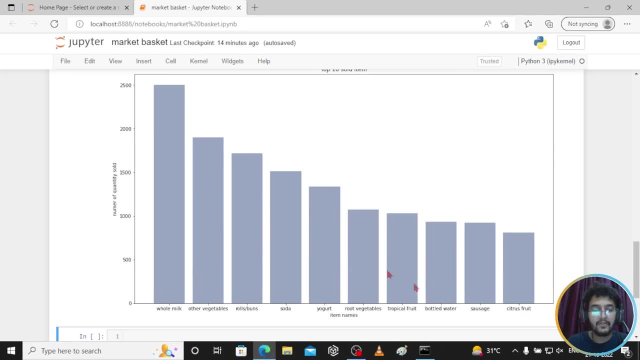 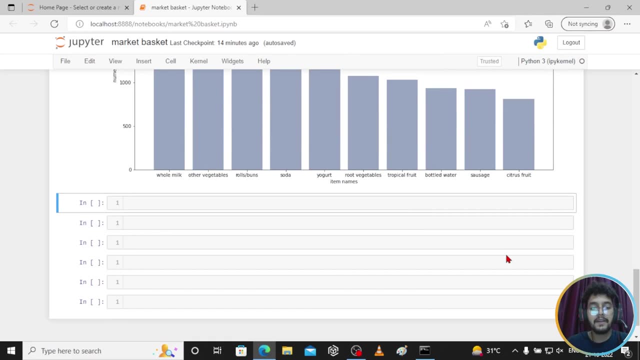 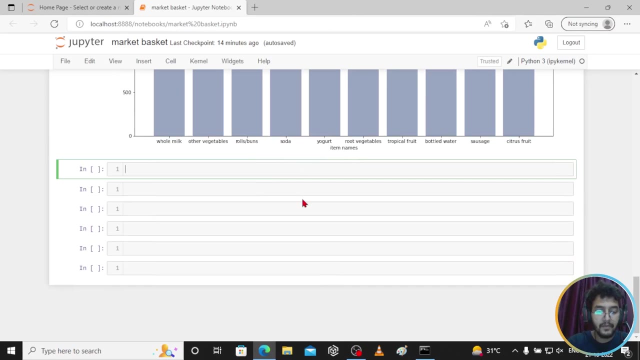 then yogurt till the citrus fruit. so these are in descending order. okay, moving forward. let's set date as index as index plotting purpose. okay, for that, i will write here. okay, let's set date as index as index plotting purpose. okay, for that i will write here here: df- underscore date. then it goes to tf dot. set underscore index date. okay, df. 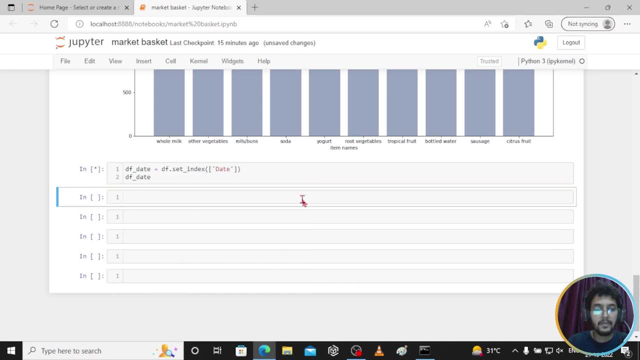 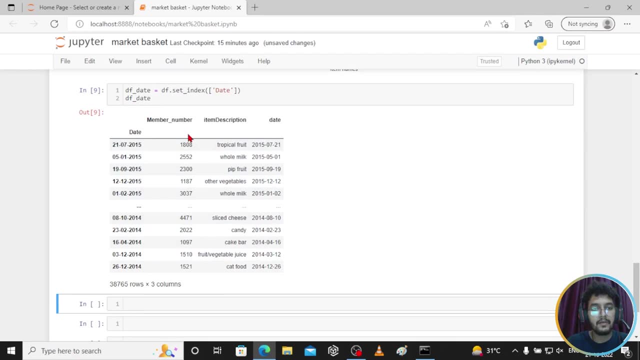 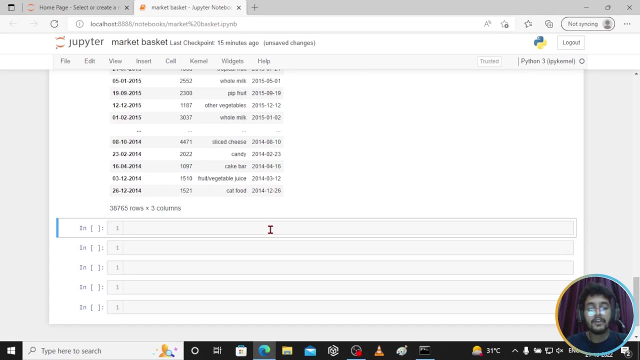 underscore date, then press enter. okay, so here you can see all the dates and the member number and the item description. okay, so date is set. so i hope you understand till here. like if you have any question or any query regarding any code or question, just put as. 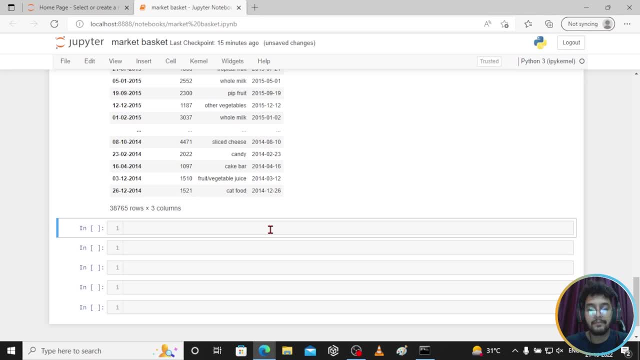 in comments. our team will shortly provide you the correct solution. okay, i'm repeating again. i hope you understand till here. if you have any question or any doubt, please comment down the below. our team will shortly provide you the correct solution. so moving forward, let's make a graph again. okay, another graph. so df: underscore, date, dot the sample. 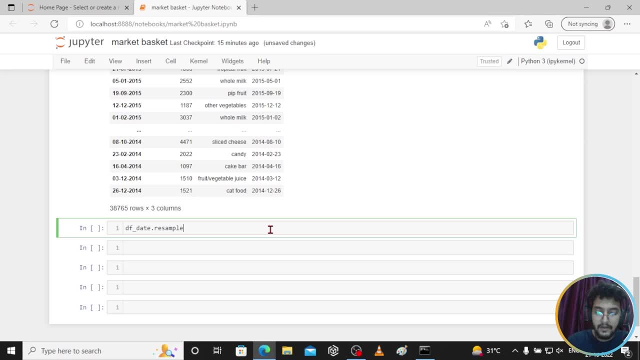 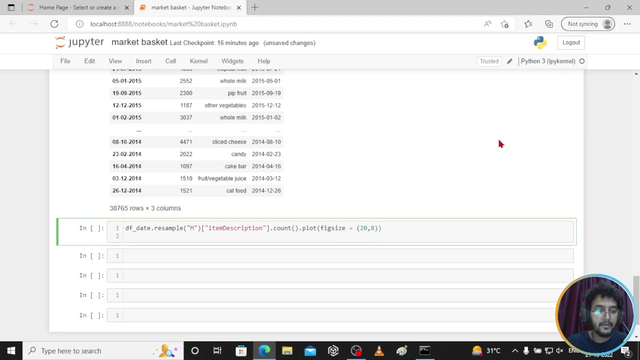 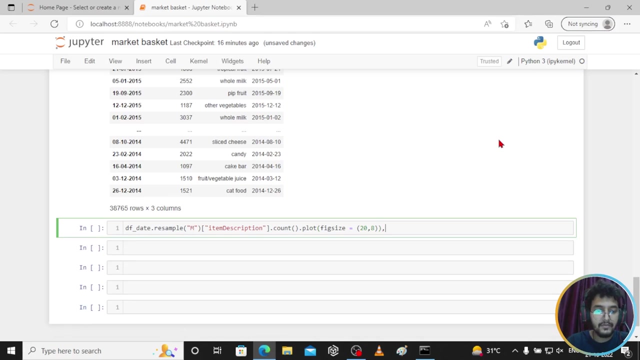 then here i will write medium m that into that outer circle. then item description. item description. point, point point 8: 8 dot plot. so let me continue here. here I will write: grid equals to true. then let me set the title: title equals to okay. number of. 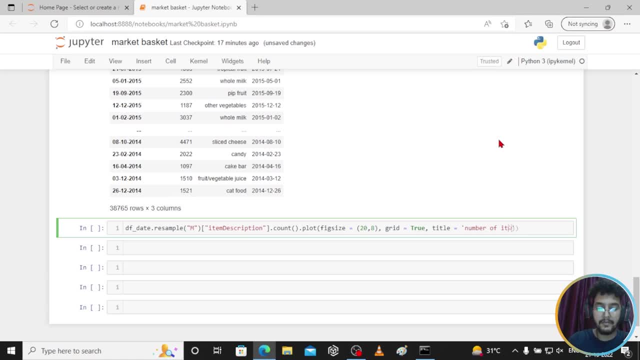 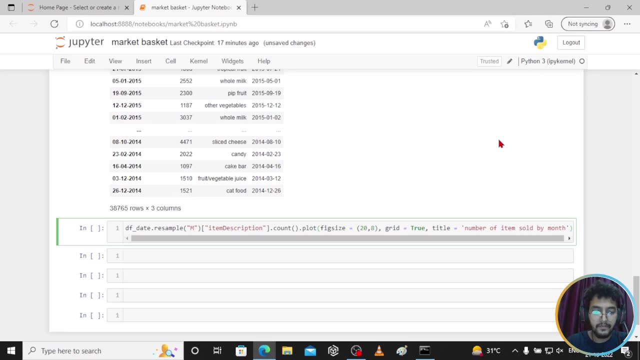 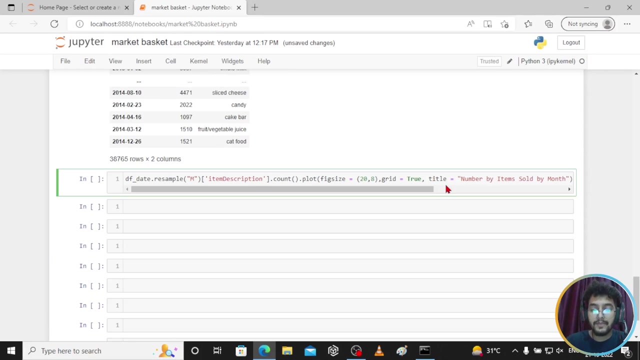 number of item sold by month. okay, then comma set, let me do dot set label. X label equals to that's good date and Y label equals to number of item sold. okay, so code is looking. okay, so let me run this. so press enter. so yeah, so here you can see the number of. 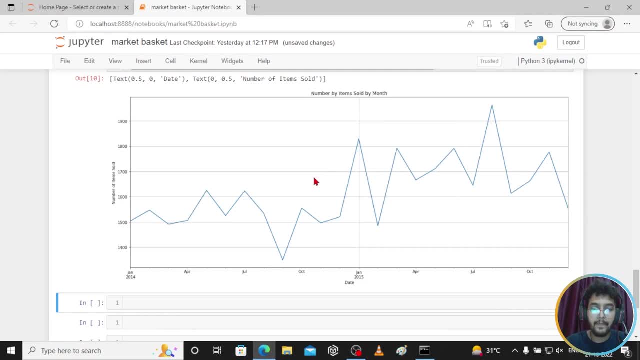 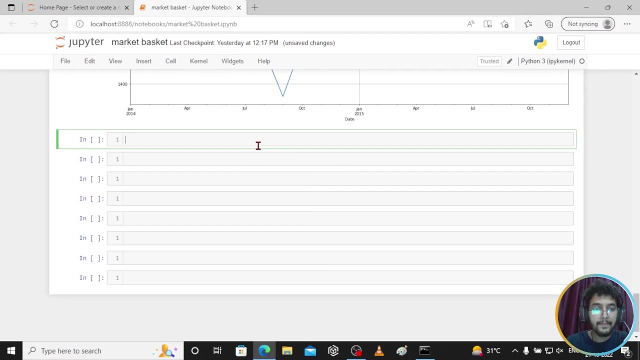 item sold by a month. okay, so you can see the graph. so, moving forward, we will select only required variable for modeling and removing white space. if any, for that I have to write here. I will write here. count, sorry, I will write here. customer level equals to dear. 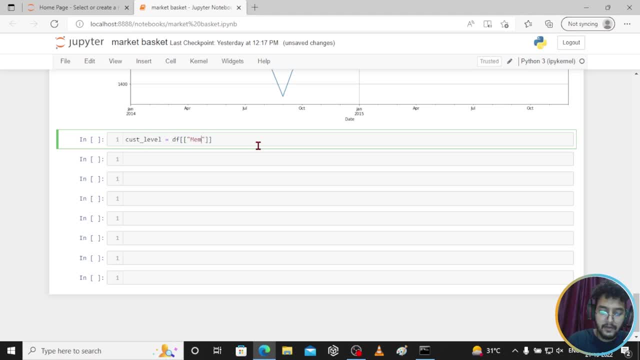 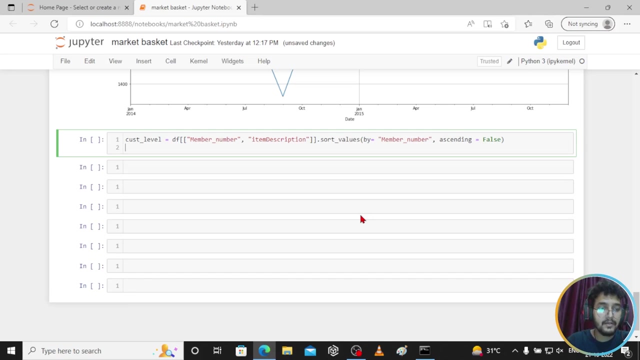 okay, then remember number, comma, item description. okay, dot. sort values by request number, so I will write here number number. okay, then comma sending question: false. then like customer level equals to, not equals to this time item description. ok, then equals to customer level, then item description str. 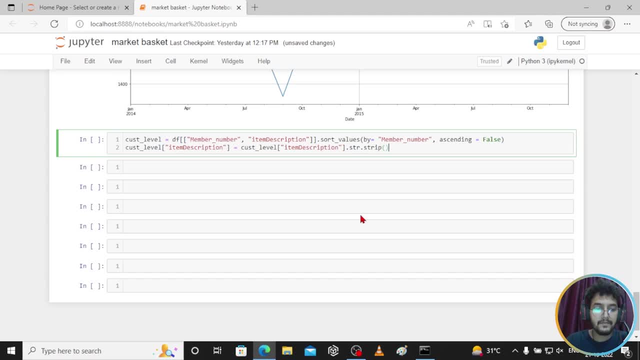 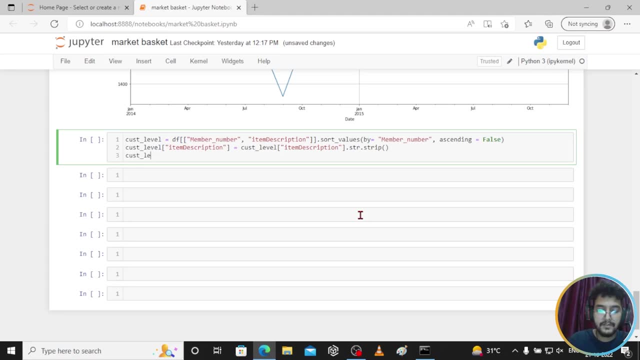 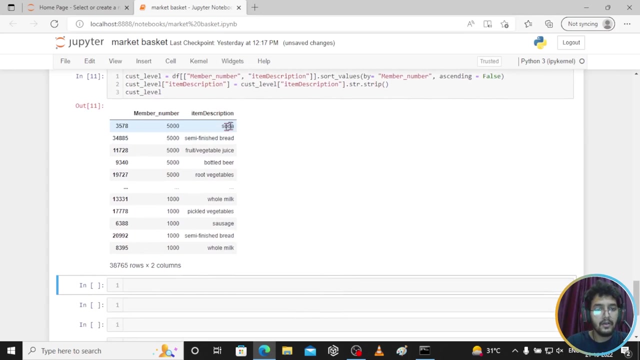 script, then customer level: ok, so press enter. so yeah, ok, so everything is good and fine. so let's move forward and combine all the items in the list format for each customer. so for that I will write here: transactions equals to a 1 for like item description. 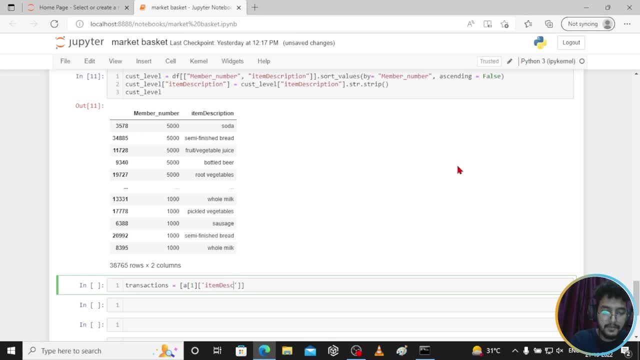 dot to list. ok, so right here I will write for a in list than 11. so right here I will write for a in list than 11. so right here I will write for a in list than 11. dot group by dot group by than here I will write. member. 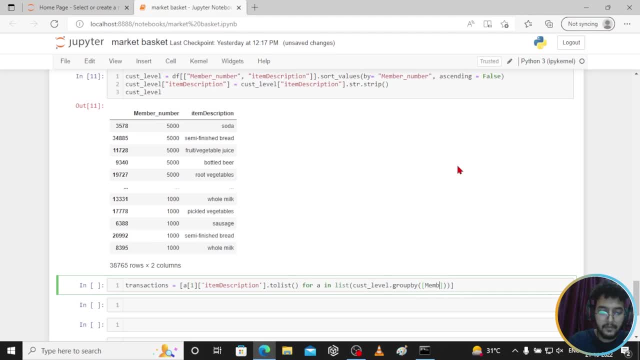 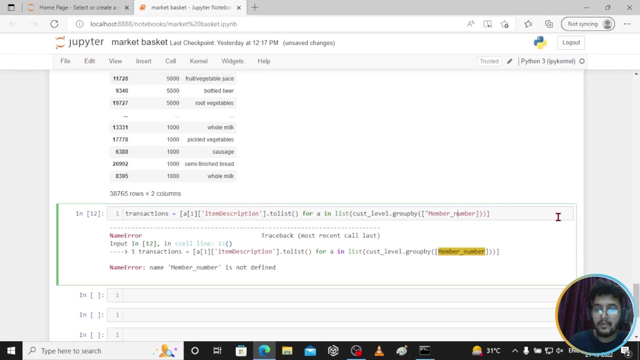 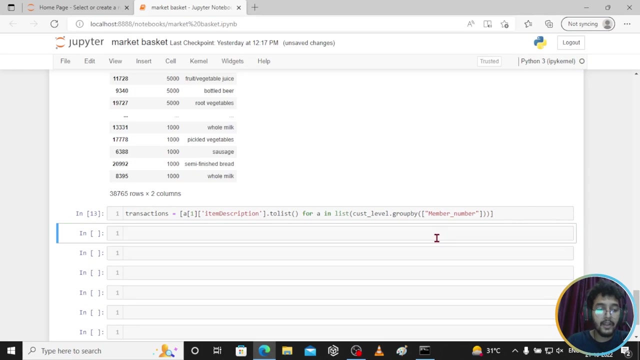 number. ok, then press enter. ok, ok, ok, sorry. ok. then press enter. ok, ok, ok, sorry, ok, ok, ok, sorry, forget, forget, forget, yeah. then press enter. so now let's import a priory package for the model creation. here I will write from apriori: import ap. 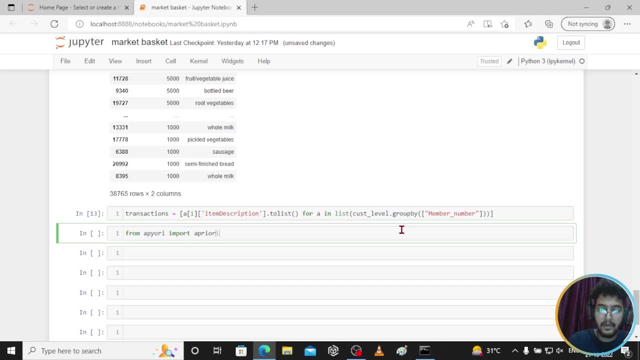 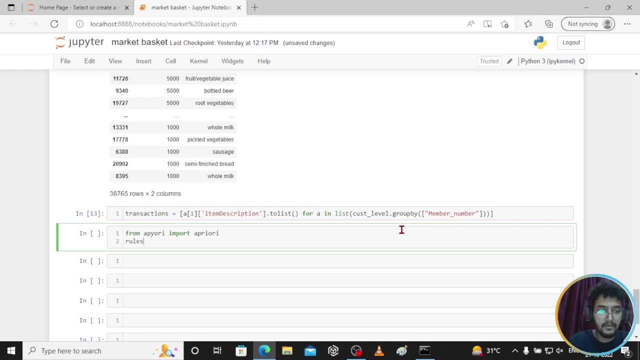 apriori. ok, so so here I will write rules: rules equals to apriori transactions. equals to apriori transactions. equals to transaction comma. like minimum support. like minimum support. equals to 0.02. ok, not 0.002. ok, not 0.002. 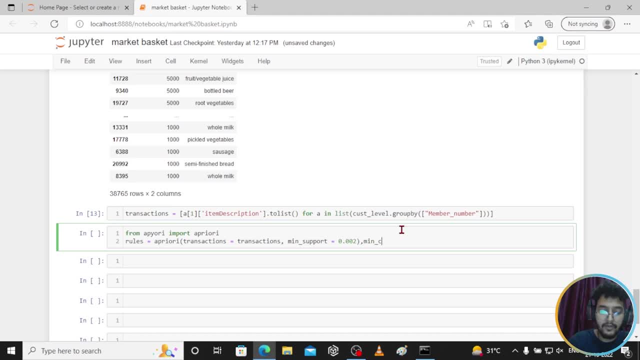 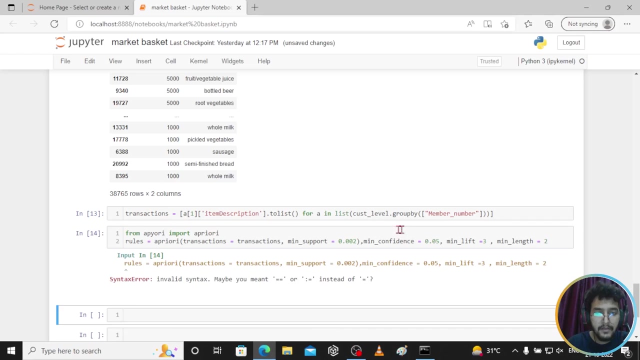 and comma, and comma. minimum confidence should be equals to 0.05. ok, then minimum lift equals to 3, equals to 3. then minimum length equals to, equals to 2. ok, so this is for the model creation. press enter. ok, rules equals to- maybe you meant equals to. 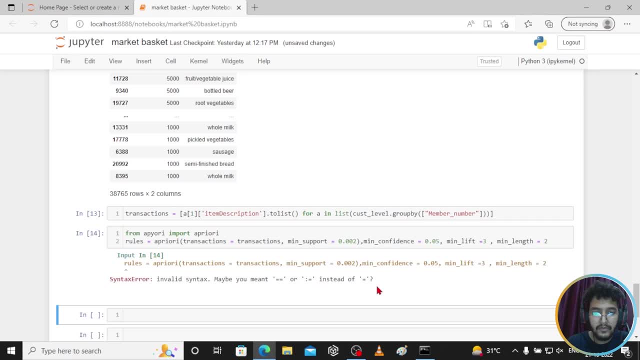 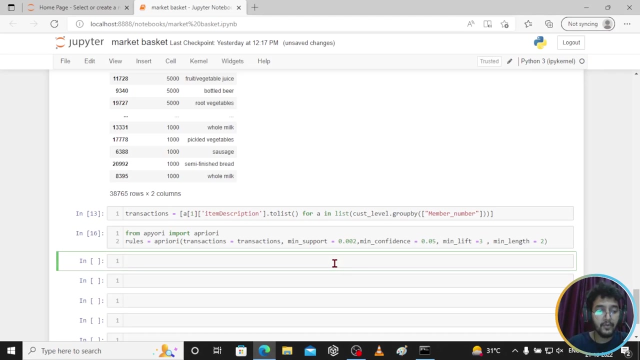 equals to instead of: ok, ok, ok, ok, ok, okay, ok, ok, ok, here's the thing, here's the thing, here's the thing, yeah, yeah. so model creation is done. so moving forward, let's store result in the less format for better visuals and let's see the results. 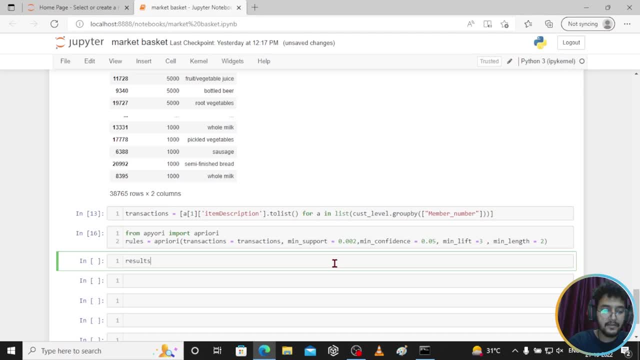 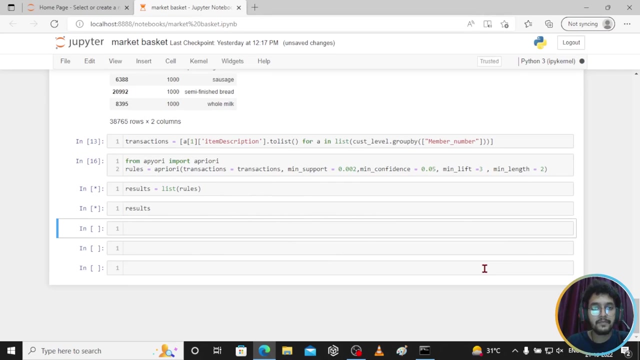 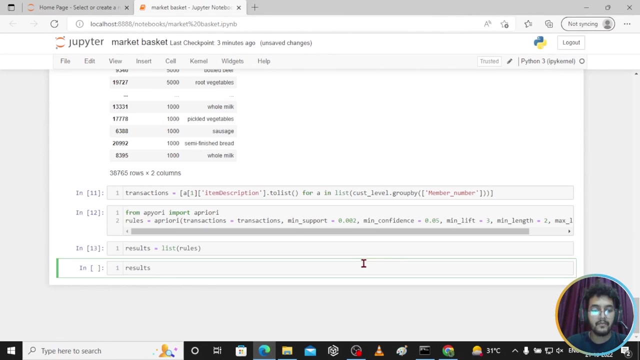 visuals and let's see the results. write results equals to list of rules and press enter. then results. press enter so it's loading, still loading. this will take some time. it's still loading, taking some time, so let me restart and run on. so press enter. yeah, so. 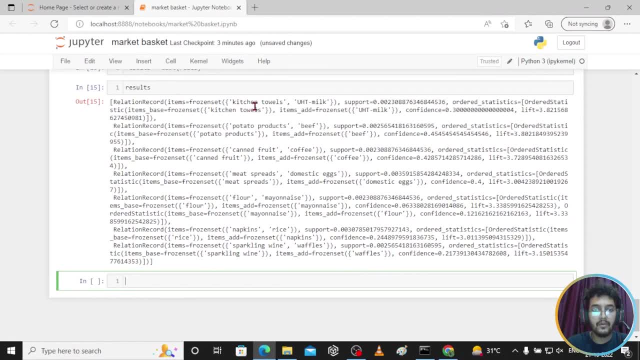 here you can see the results. so now i repeat: so like kitchen towels, like usd milk and potato products, beef meat spreads, dramatic x. so these are the some examples. so moving forwards, creating user defined function for arranging the results okay, in proper manner. so obtain from model and readable. 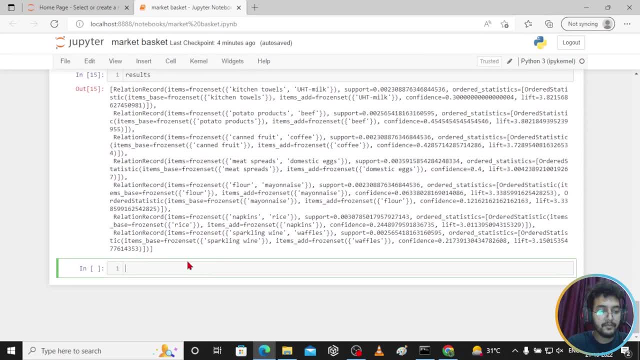 format. so here i will write for that df also inspect results. okay, for that lts equals to tuple, then results, then two zero, then again zero. okay, so here i will write zero again for result, for result, end results, then rhs. sorry, rhs equals to. let me copy from here: 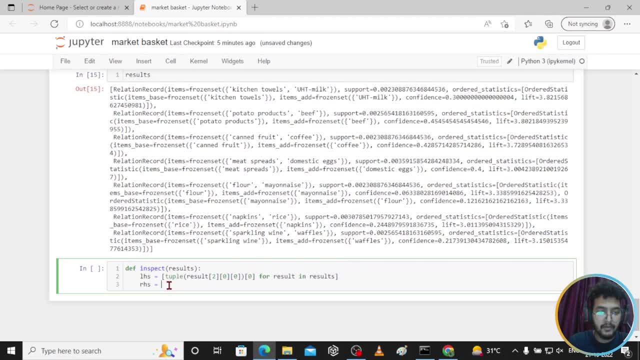 let me copy from here and i will make the edits: okay. instead of zero i will put here one, okay, then supports a question. so results: result one for result and result. so now confidence: result two. result two. result two: zero two. uh, four results in results: result two. 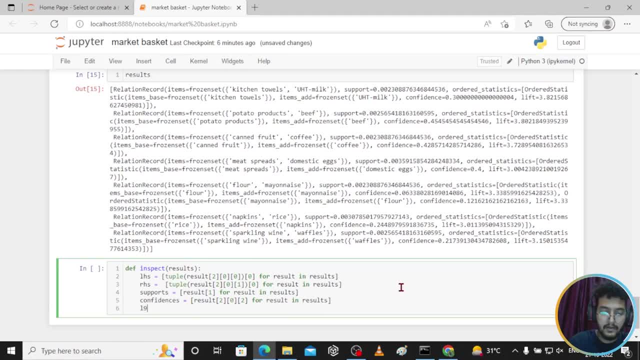 and Nets equals result two, three and time for left of result. as your Jazz, this example results two. tried before forgetting the time: result two, then 0,, 3,, 4, Result: End Results. okay, then lift is complete. then I will write return List Zip: LHS, RHS Supports Confidence, Confidences, Lift. 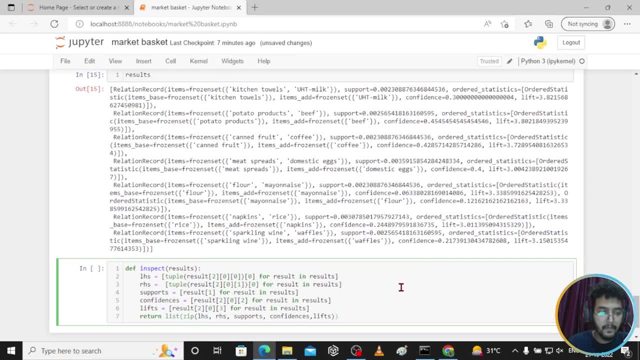 Lifts. okay, then I will write here Result Results in DataFrame. goes to pdDataFrame: inspect Results. comma Column goes to Left-hand side: okay, comma, then right-hand side. Okay then. comma support, then comma confidence, confidences, comma lift. 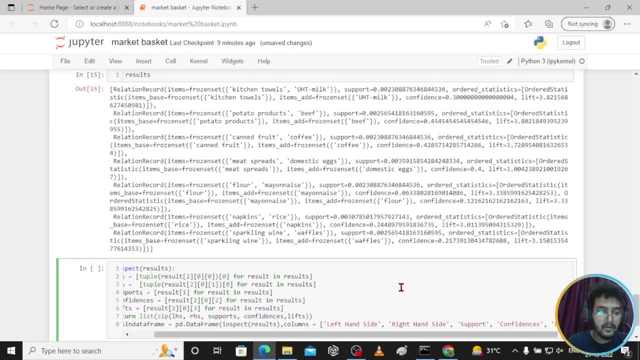 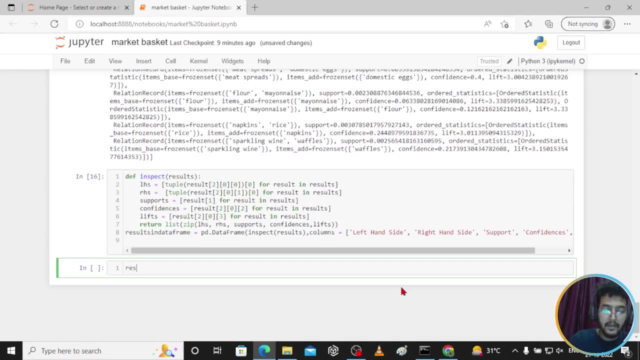 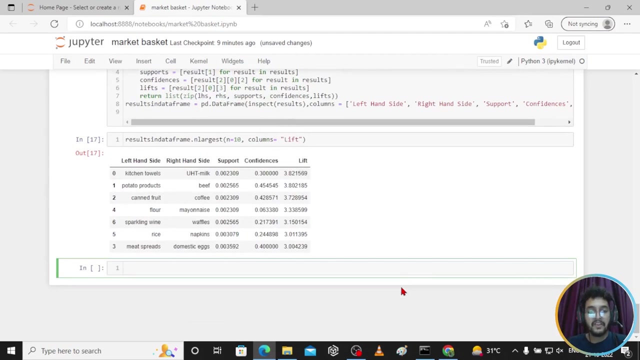 Okay, press enter. so now I will run it. so here I will write result in data frame. okay, f is small, dot n largest, n largest, Then n equals to 10, comma columns pursue: lift: okay, yeah, so here you can see the. 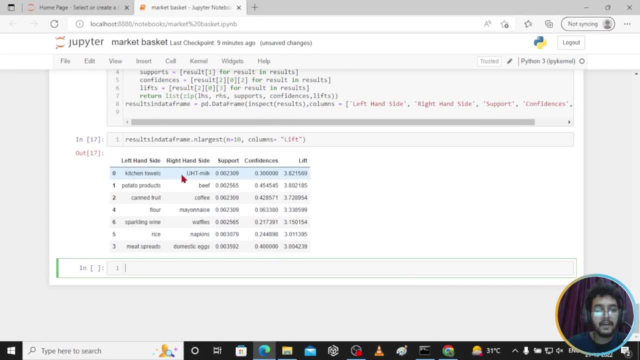 the best possible scenarios. okay then, kitchen towels, UST milk. these are the some recommendation when the customer will buy this, So these are the recommendation that he or she also buy this. Okay, so I hope you are understand till here. if you have any questions or any query regarding, 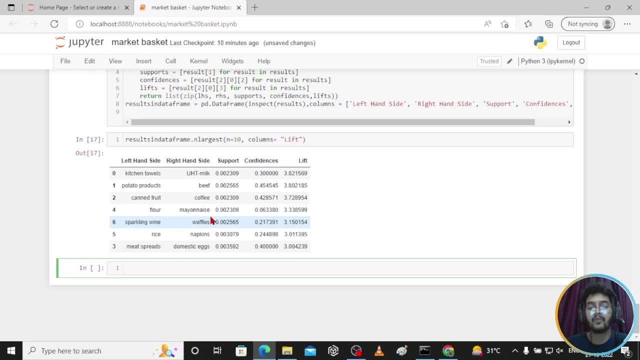 any code or question, just put as in comments. our team will shortly provide you the correct solution. I hope you guys must have understood how you can do market based basket analysis using Python. If you have any queries, you can ask in the comment section below. our team will respond.